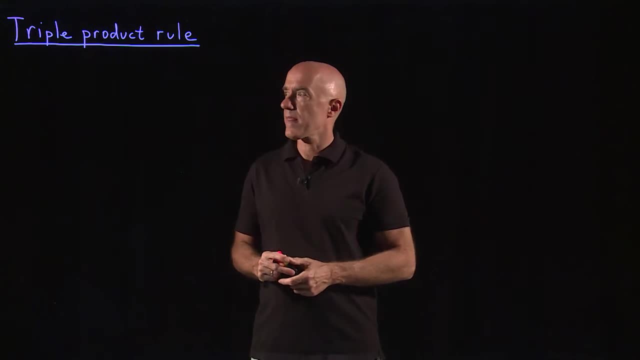 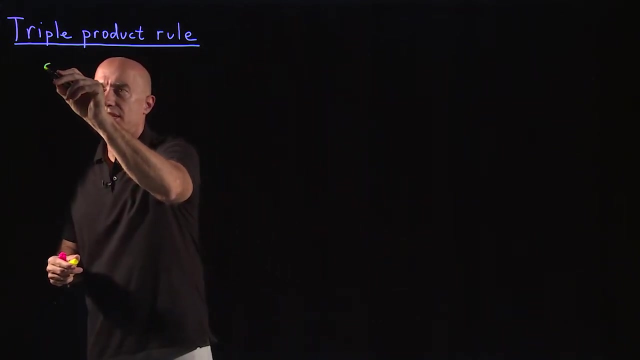 you an example using the ideal gas law. Okay, so what is the triple product rule? We assume we have three variables, and I'll call them x, y and z, but they're related, So you can write then a function f of x, y. 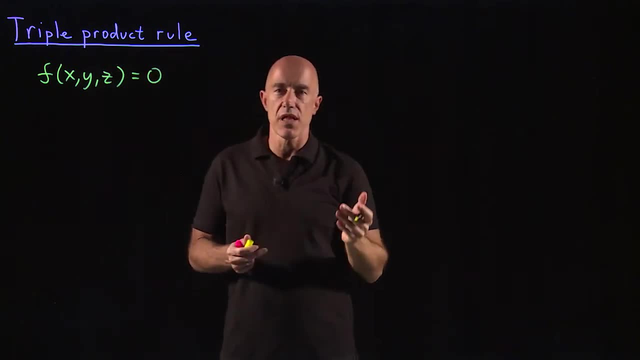 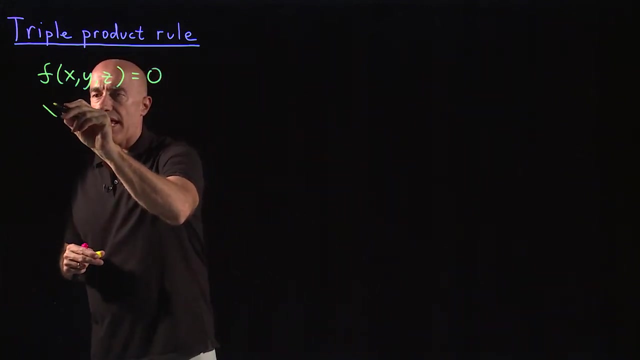 z equal to zero. So that gives you the relationship between the three variables x, y and z. Since they're related, you ought to be able to solve for x or solve for y or solve for z. So, for instance, you can write x, which is a function of y and z, or you can write: 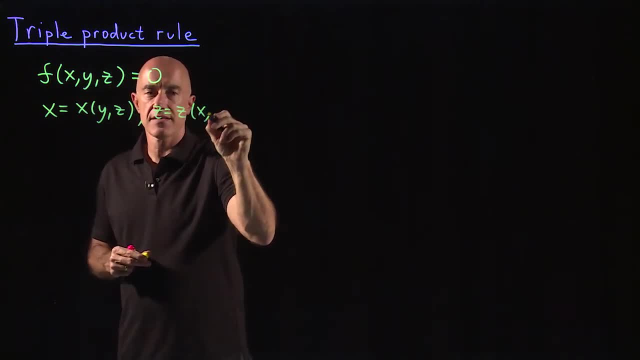 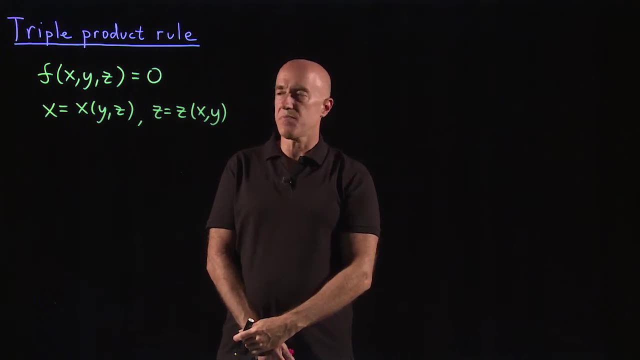 z as a function of x and y. Okay, Let's take the differential of these expressions using the partial derivatives, like when we did the triple product rule. Let's take the differential of these expressions using the partial derivatives, like when we did the triple product rule. Let's 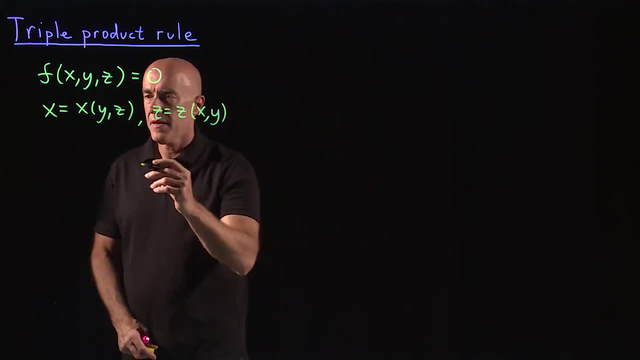 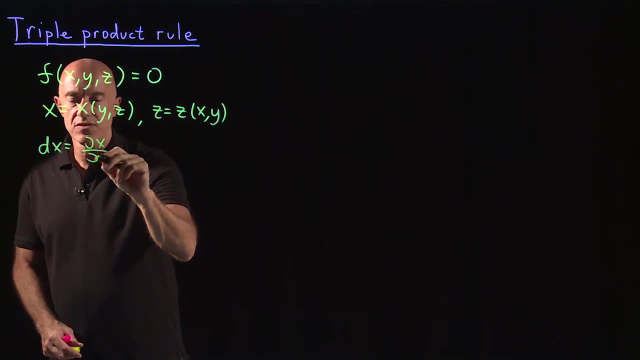 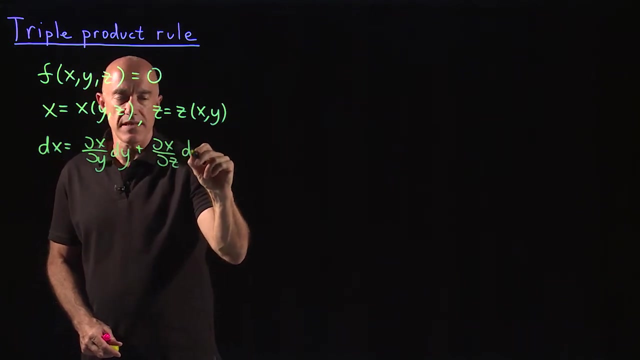 take the differential of these expressions using the partial derivatives, like we did in the lecture on the chain rule. So we have the differential: dx is equal to the partial of x with respect to y times dy, plus the partial of x with respect to z times dz. Okay, 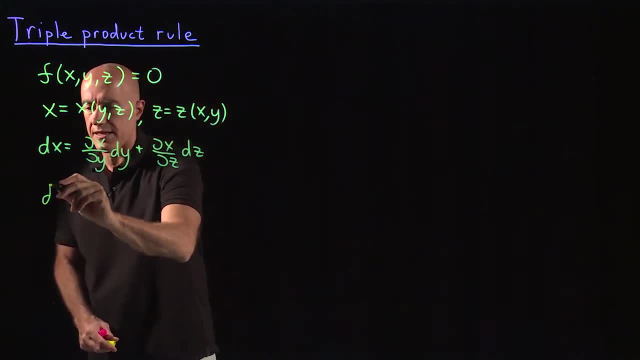 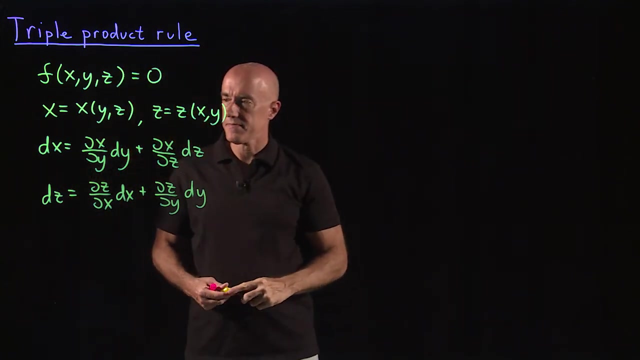 And then we also have the differential of z. dz is equal to the partial of z with respect to x dx with respect to x dx. Thanks, plus the partial of z with respect to y dy. okay, All's good, I think. 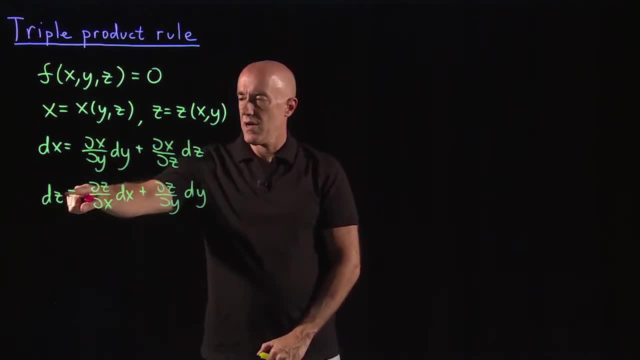 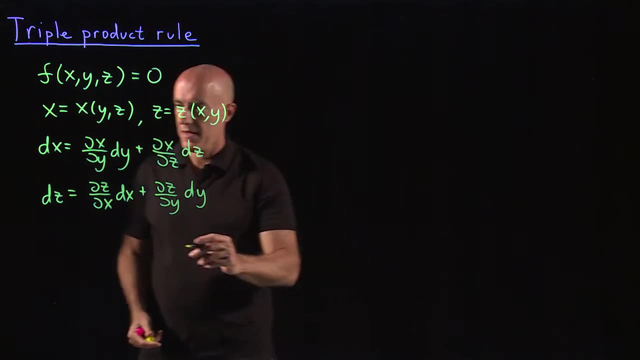 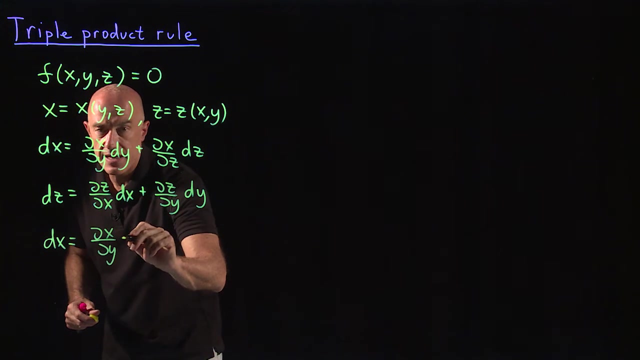 Now what I want to do is to eliminate dz from this first equation using the second equation. okay, Because I don't want dx, dy, dz. I only want to have two variables. So if we do that, we end up with: dx equals partial of x with respect to y, dy. 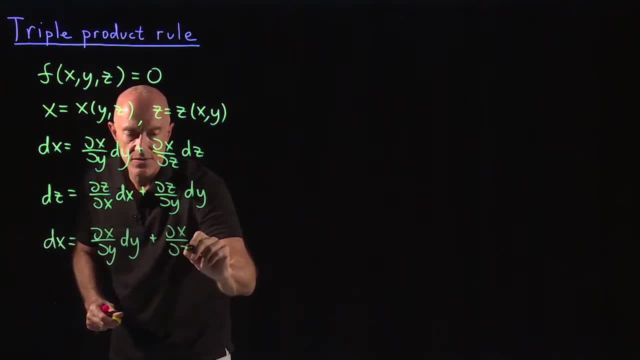 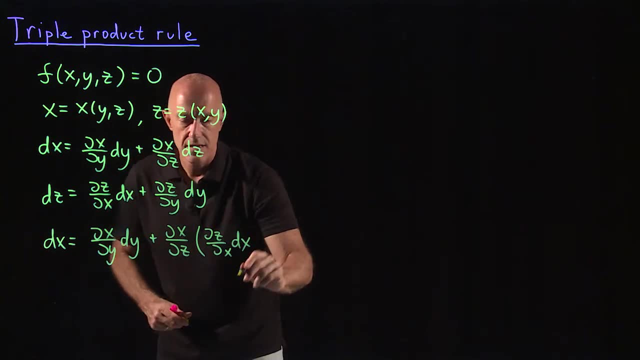 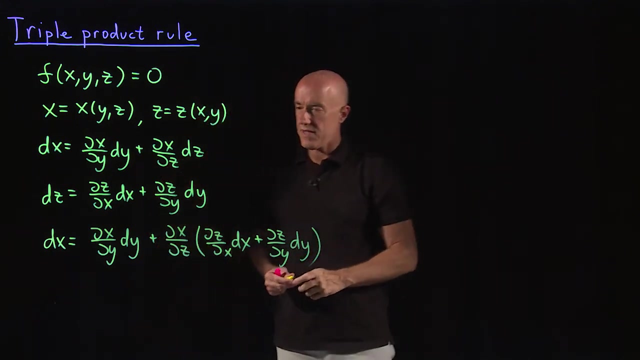 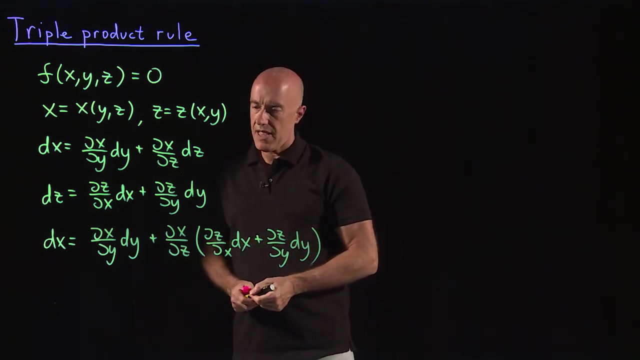 plus partial of x with respect to z times dz, which is partial of z with respect to x. dx plus partial of z with respect to y dy. okay, The next obvious thing to do is to group the dx terms and the dy terms on the same side. 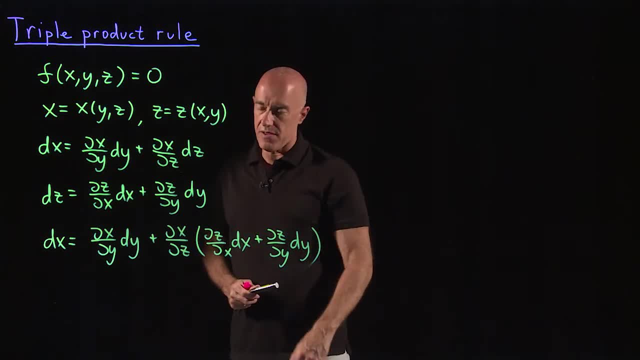 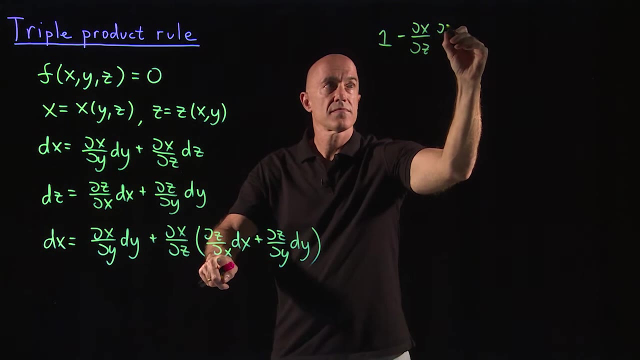 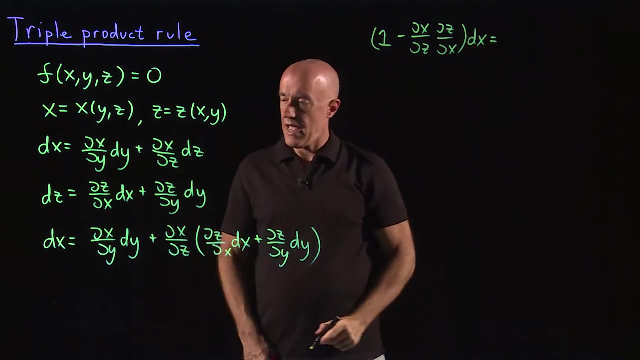 So if we put the dx on the left side and the dy on the right, the dx will end up with a 1 here and then minus dx, dz, dx, times, dx, And then we have the dy on the right, so we have dx dy. 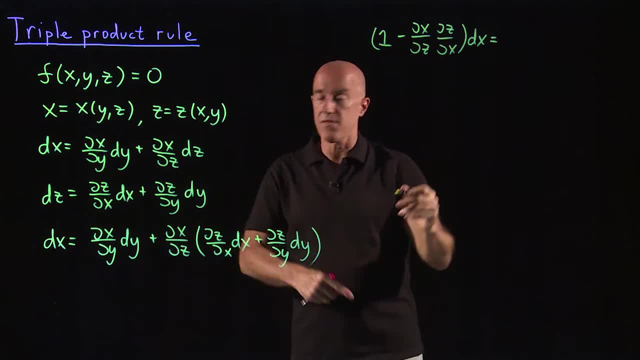 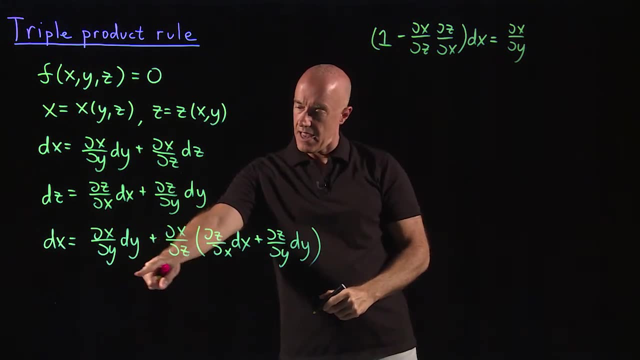 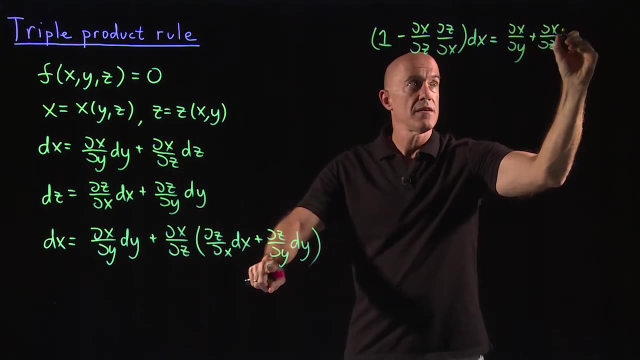 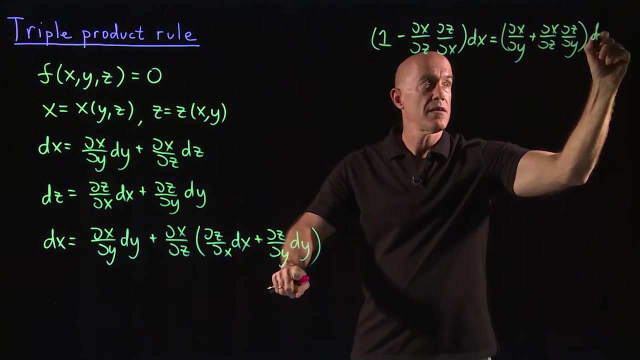 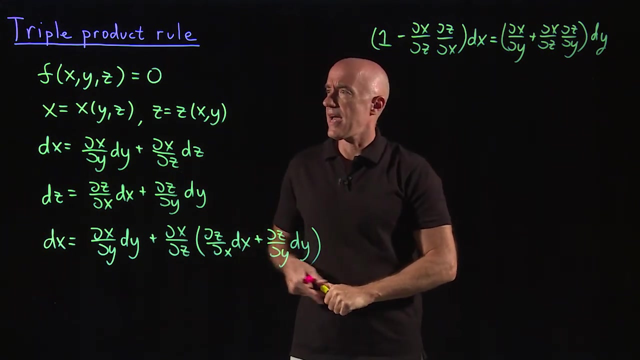 We put the dx on the left, the dy on the right, so we have dx dy here, And then plus dx, dz, dz dy, plus dx, dz dz dy, And that's multiplied. Okay. Now the key here is that we have x, y and z variables with one relationship between them. 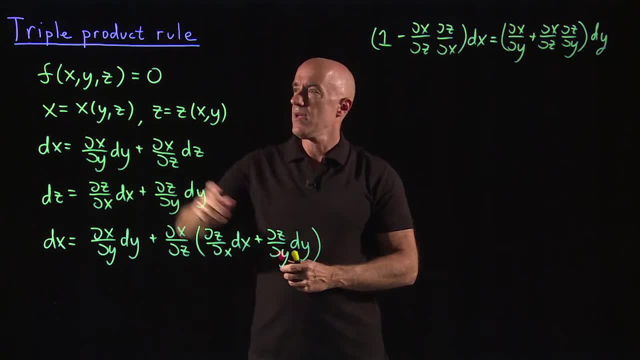 given by this function of x, y, z equals 0.. Because there's only one relationship. it means we can vary two of these variables independently. okay, We can vary any two of these variables independently. So that means we can vary x, y, z and z. 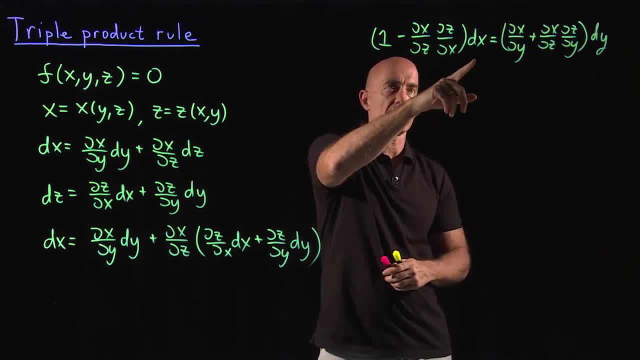 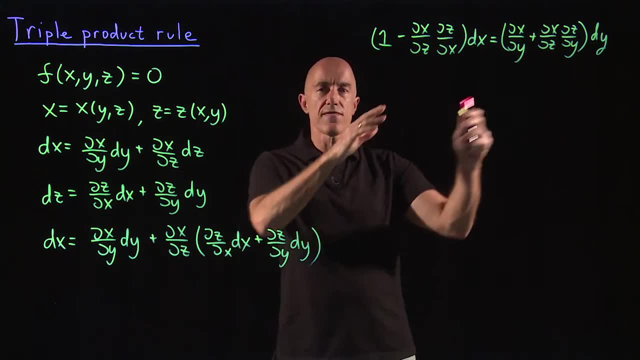 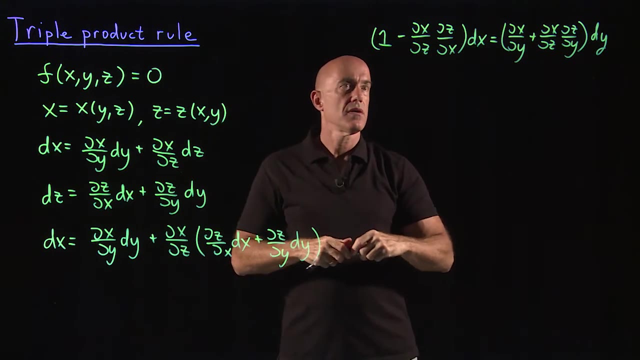 We can vary x independently, We can vary y independently, So dx and dy are independent variables that can take any values. So in order for this equality to hold, the terms in the parentheses must be 0.. Okay, So let's start with the first term in parentheses. 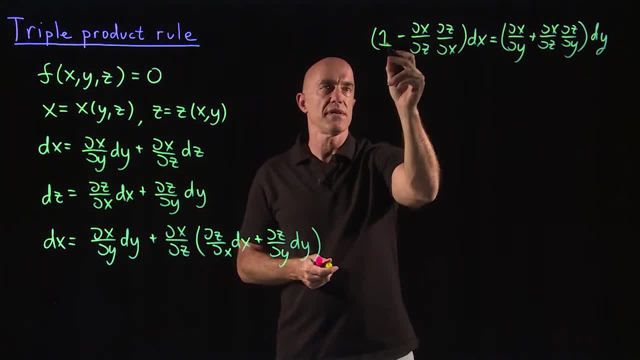 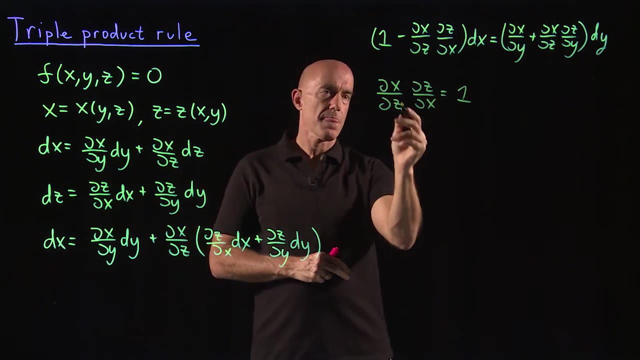 So that means dx, dz, dz. dx is supposed to be equal to 1.. Okay, So dx, dz, dz. dx equals 1, in order for the first parentheses to be 0.. This means that dz. dx is the multiplicative inverse of dx, dz, right. 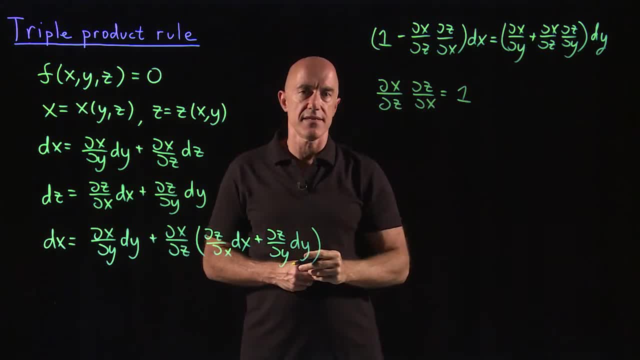 So dz- dx is 1 divided by dx, dz. That makes a lot of sense, right? You change the numerator, You flip the numerator and the denominator and it's the reciprocal Okay. So that's a relationship that makes sense to us. 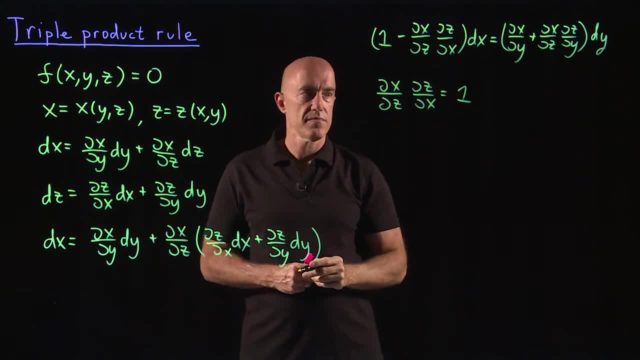 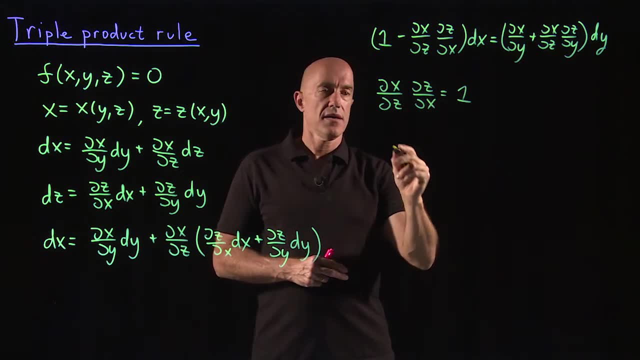 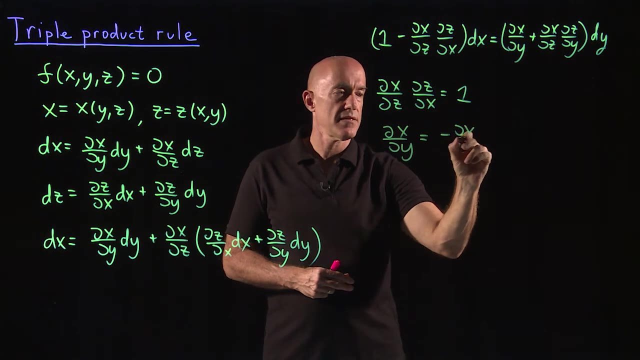 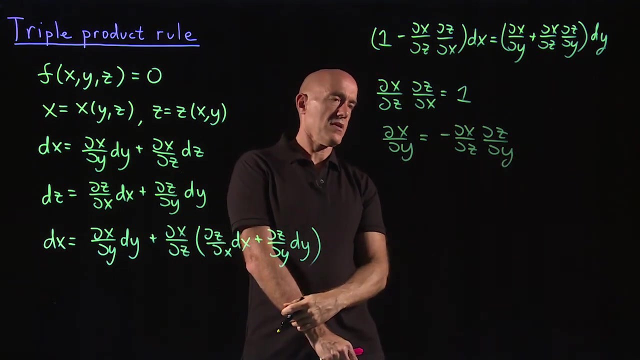 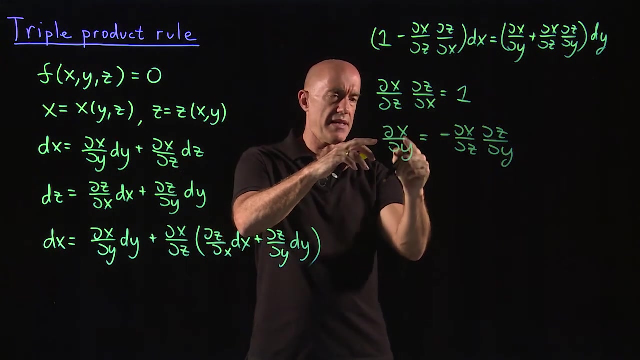 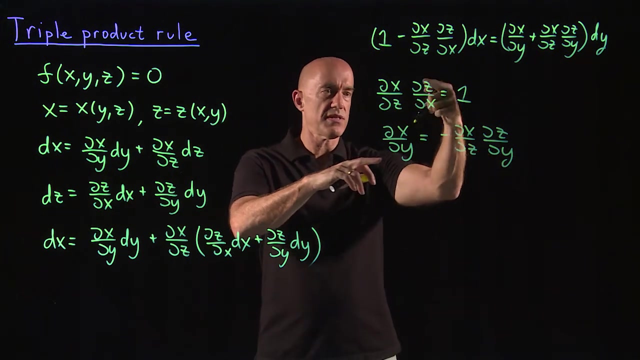 dx, dz, dz. dx equals 1.. Okay, What about the second relationship? The second relationship says dx dy is equal to minus dx, dz, dz dy. Okay, But let's put everything on the same side, So we have a dx dy To put the dz dy on the left. we can use this first identity and take the reciprocal. 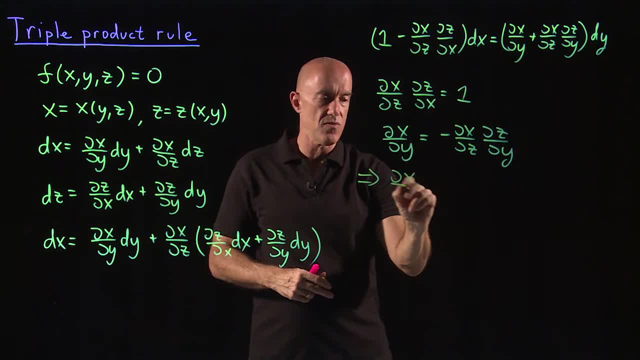 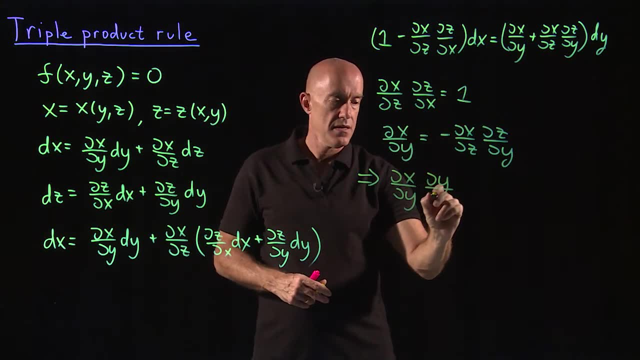 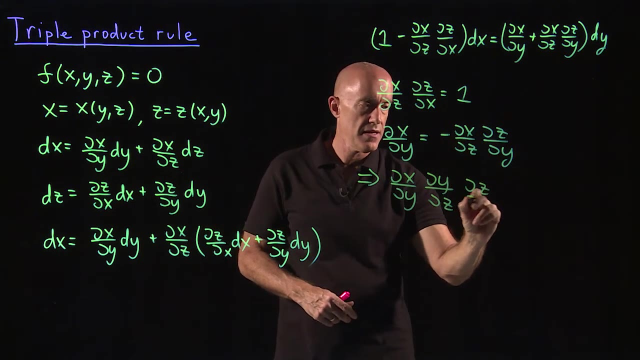 So this one is equivalent to dx dy. We move the dz dy to the left, It becomes dy dz, So dy, dz. And then we move the dx dz on the right to the left, So it becomes dz dx, And what we have left is a minus 1.. 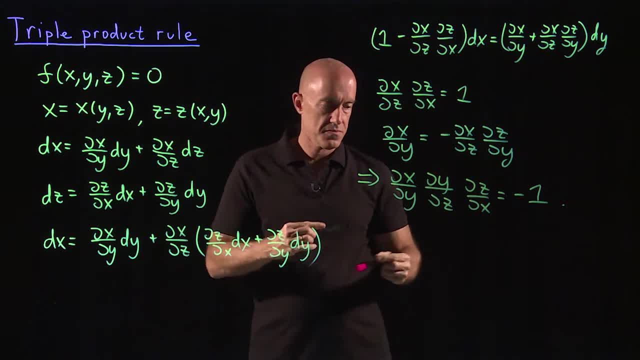 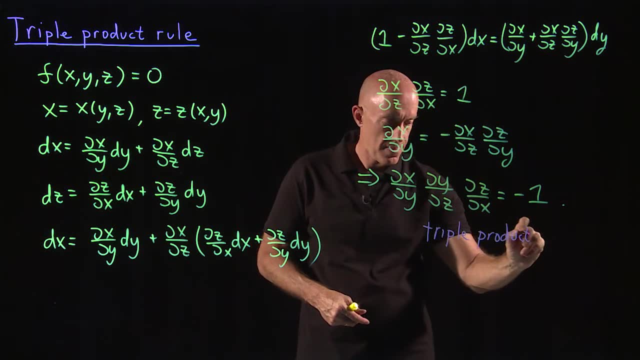 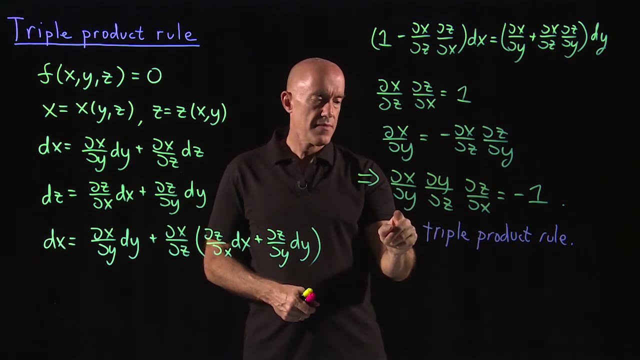 That's called the triple product rule. Okay, This is the triple product rule. Okay, Let's see, Let's look at that carefully. dx dy- Notice the y matches. dx, dy, dy, dz. Notice the z matches: dz, dx. 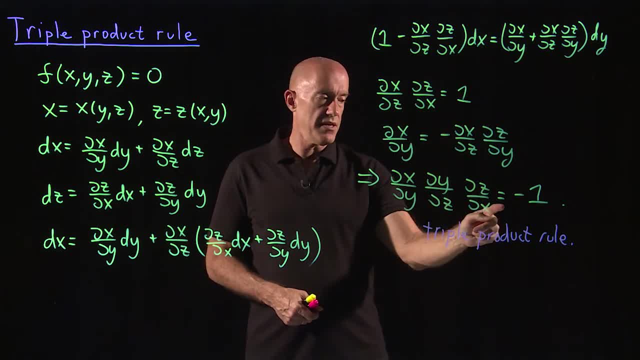 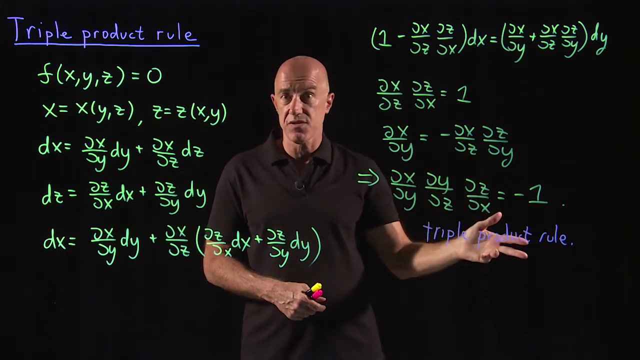 dx, dy, dy, dz, dz, dx equals minus 1.. Minus 1.. That always amazes me, You know. I mean, if these were normal derivatives, derivatives of function of single variable, you would be very happy to cross out dy, dy, dz, dz, dx, dx and get plus 1.. 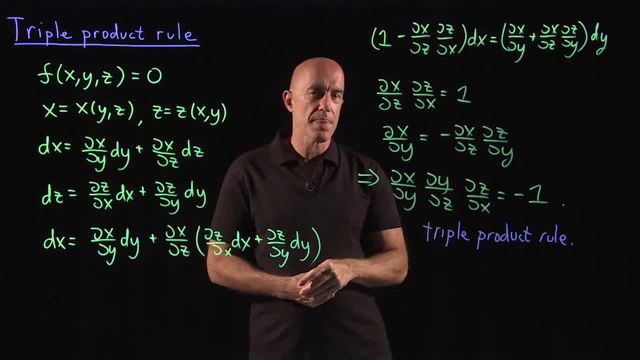 But partial derivatives don't work that way. Partial derivatives are not delta x divided by delta y like a single variable derivative. They behave differently. So this triple product rule: you don't get plus 1,, you get minus 1.. Okay, 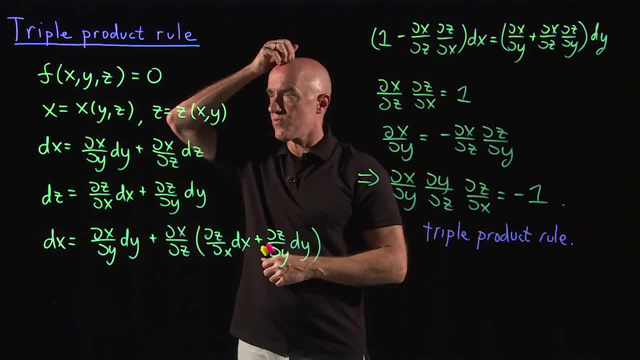 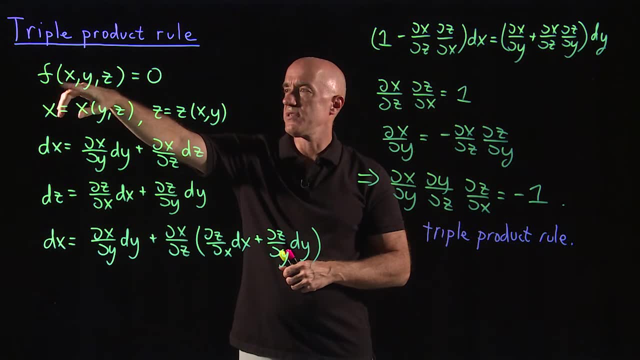 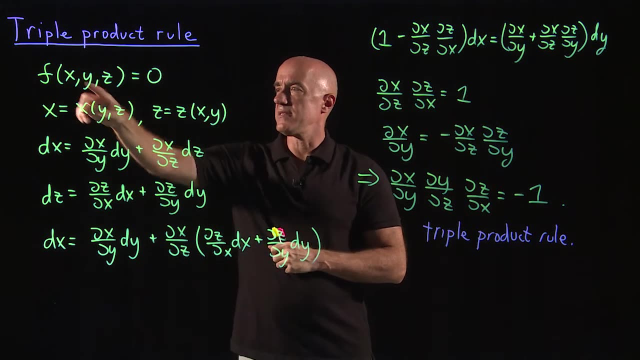 Let me review. So the triple product rule is when you have two variables that have a single relationship and you can write that relationship, say, as f of x, y, z equals 0. We didn't actually use that formula, But what it means is that you can solve for x. so x is a function of y and z.